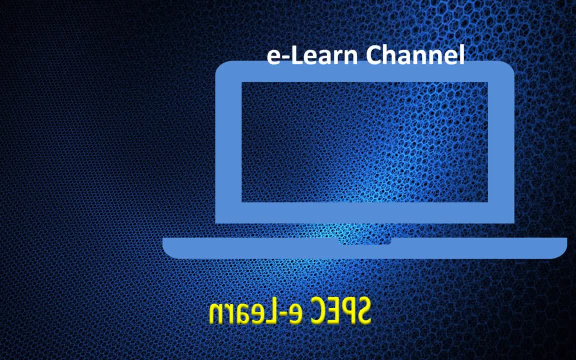 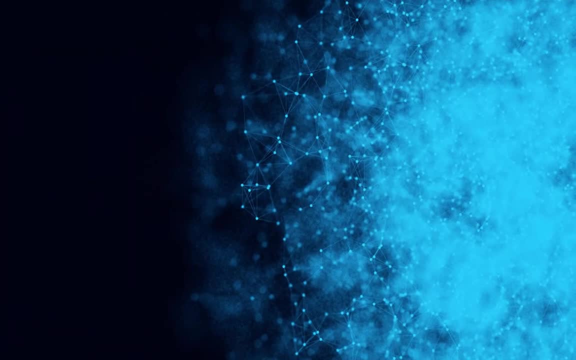 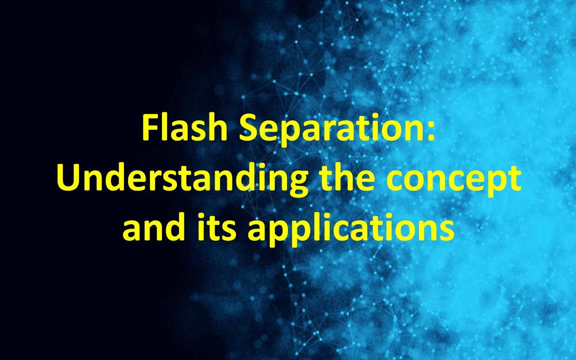 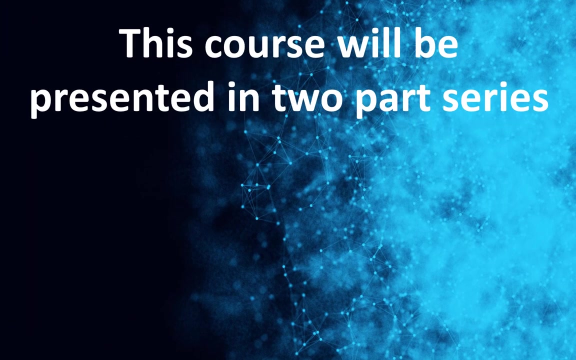 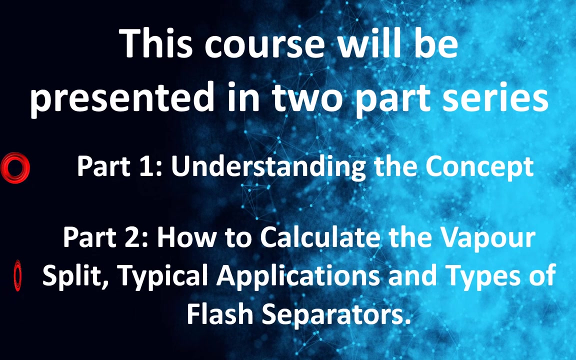 Hello everyone, welcome to SPECT eLearn, the online learning channel dedicated to chemical engineers. Flash Separation: Understanding the Concept and its Applications. This course will be presented in two part series: Part 1, Understanding the Concept. Part 2, How to Calculate the Vapour Split: Typical Applications and Types of Flash Separators. 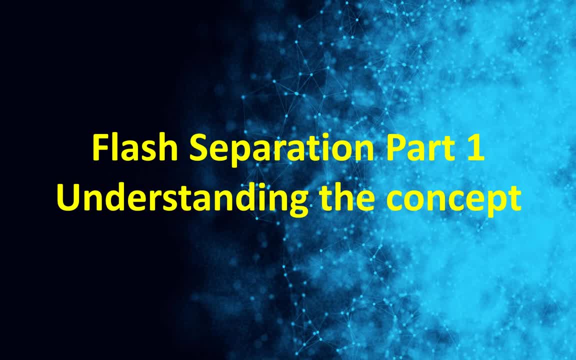 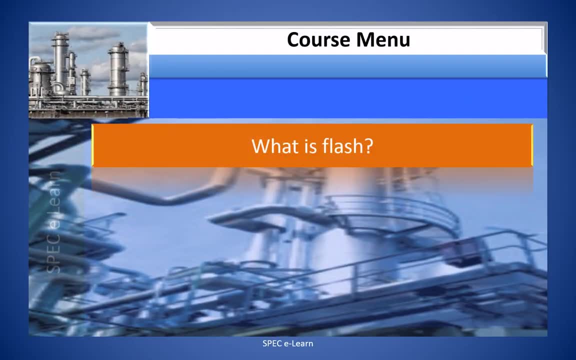 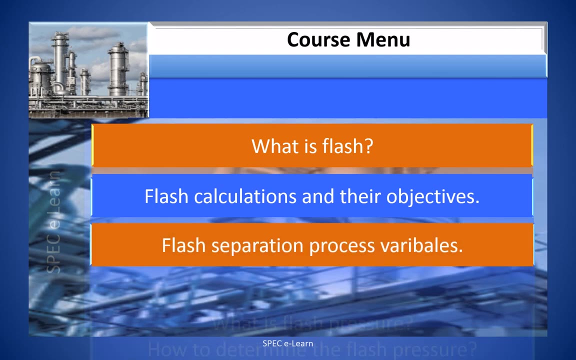 Flash Separation- Part 1, Understanding the Concept. In this part 1 of the video, you will learn what is flash, flash calculations and their objectives. flash calculations and their objectives. flash separation process variables. what is flash pressure and how to determine the flash pressure. 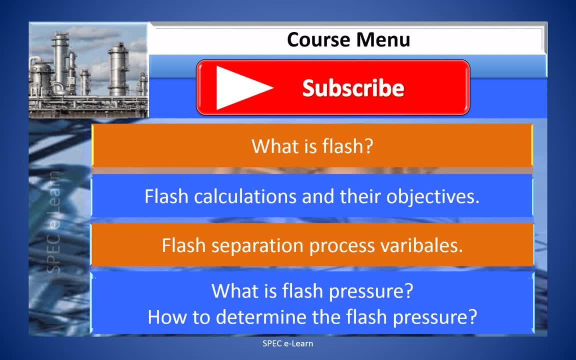 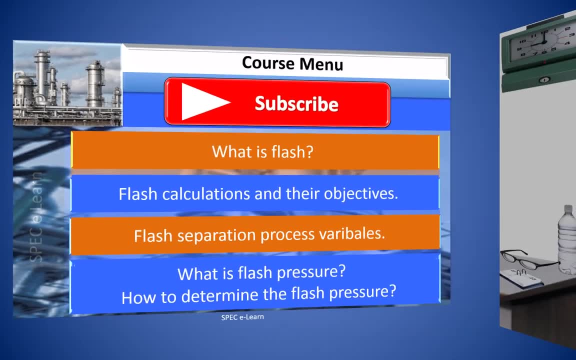 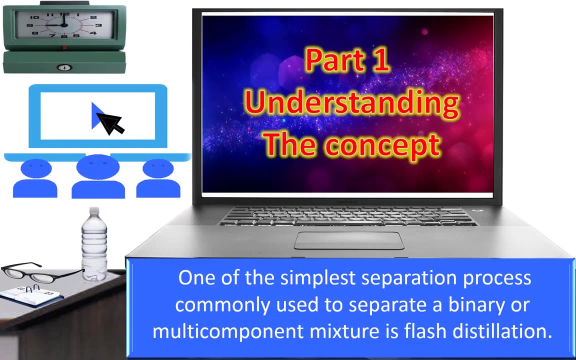 Please subscribe to the channel. By subscribing, you will motivate us to produce knowledgeable video content for you. So subscribe now, before you forget. One of the simplest separation process commonly used to separate a binary or multi-combinant mixer is flash distillation. 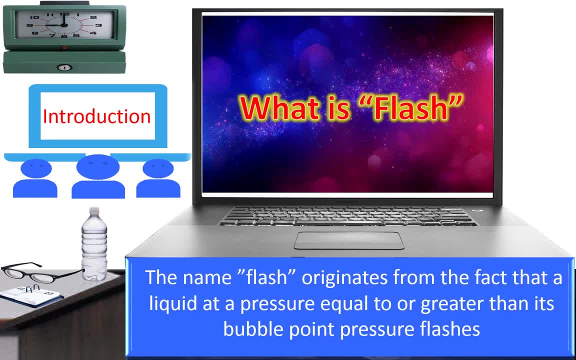 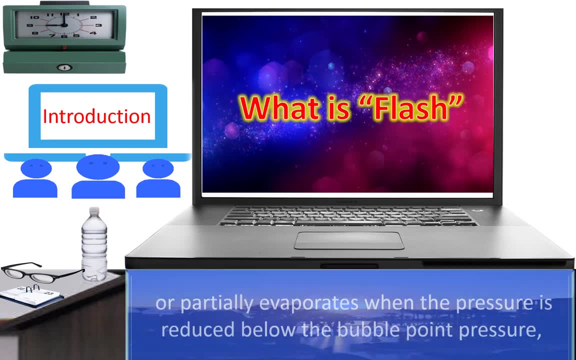 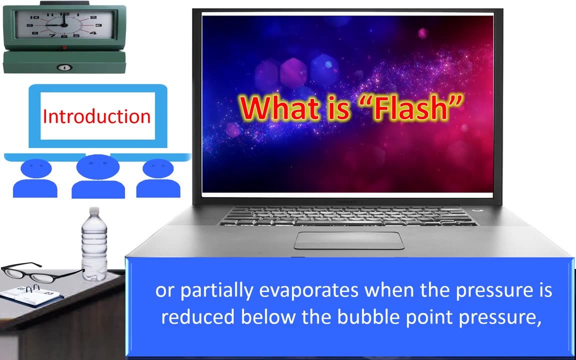 The name flash originates from the fact that a liquid at a pressure equal to or greater than its bubble point pressure flashes or partially evaporates when the pressure is reduced below the bubble point pressure, producing a two-phase system of vapour and liquid in equilibrium. 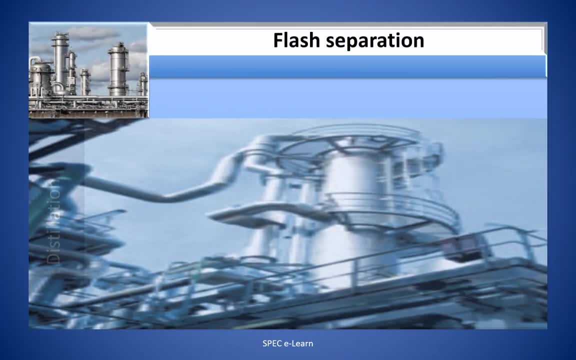 Flash Delivers the Calculations of Attacking and Dude Glides. So flash Wrong Lambda Analysis. that proposes a two-phase system of vapour and liquid equilibrium. So flash is an equilibrium by which reaction is a difficult. that is the random Culinization system. 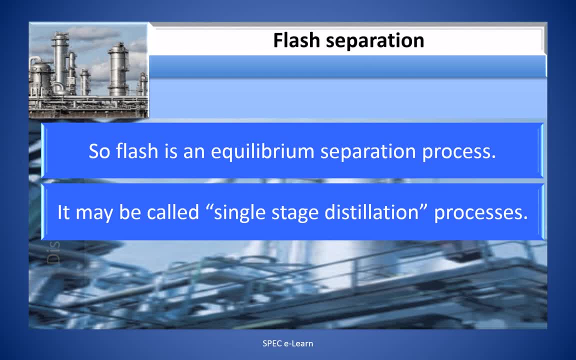 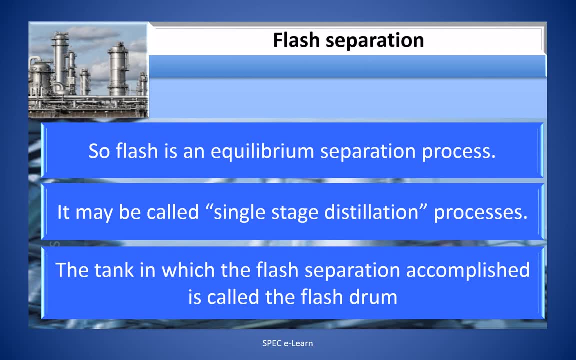 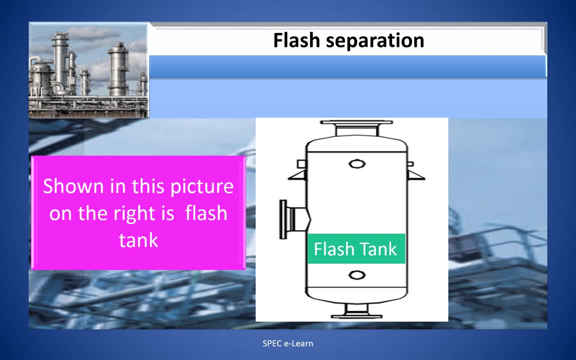 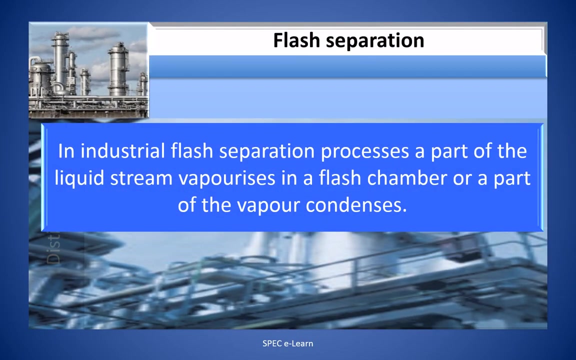 Flash is an equilibrium separation process. It may be called a single stage distillation process. The tank in which the flash separation is accomplished is called the flash drop. Shown in this figure on the side is a picture of a flash tank. In industrial flash separation processes, a pot of the liquid steam vaporizes in a flash. 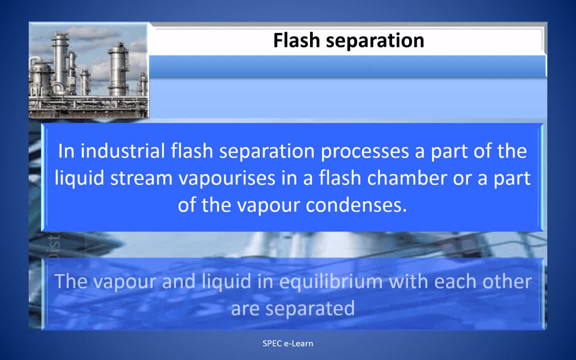 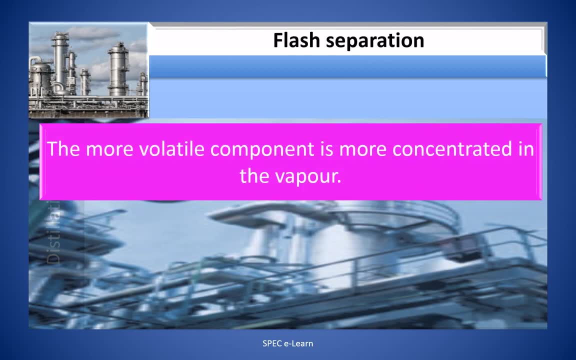 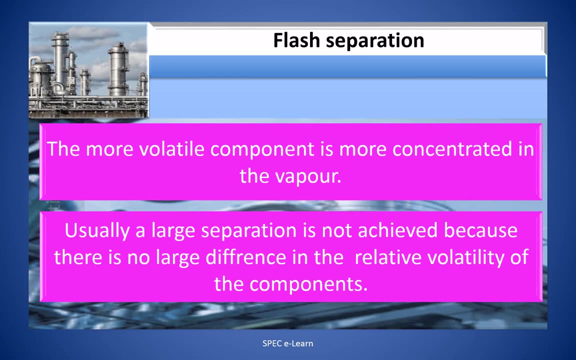 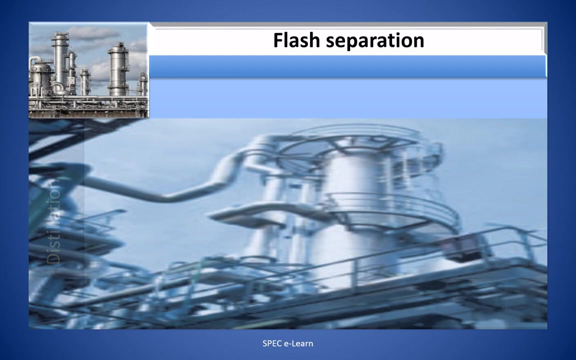 chamber or a pot of the vapor condenses The vapor and liquid in equilibrium with each other are separated. The more volatile component is more concentrated in the vapor. Usually, a large separation is not achieved because there is no large difference in the relative volatility of the components. 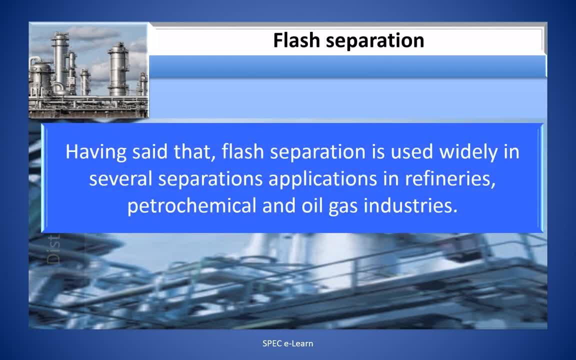 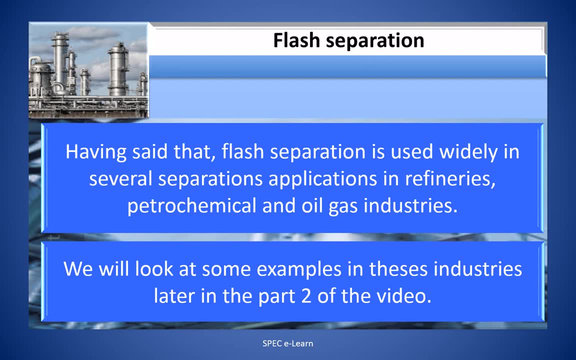 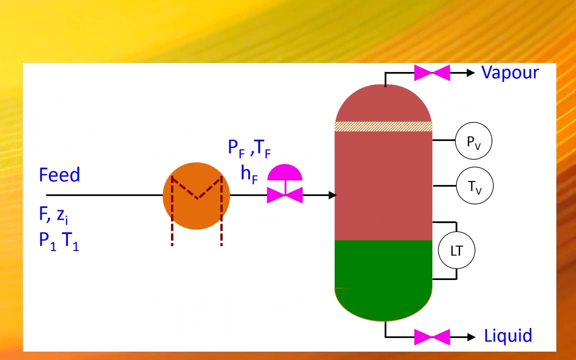 Having said that, flash separation is used widely in several separation applications in refineries, petrochemical and oil gas industries. We will look at some of the examples in these industries later. in the part 2 of the video Illustrated in this figure is flash distillation. 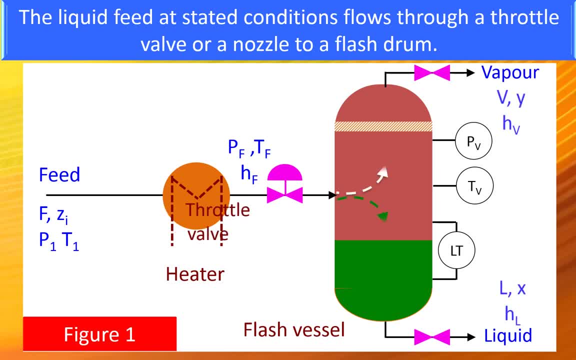 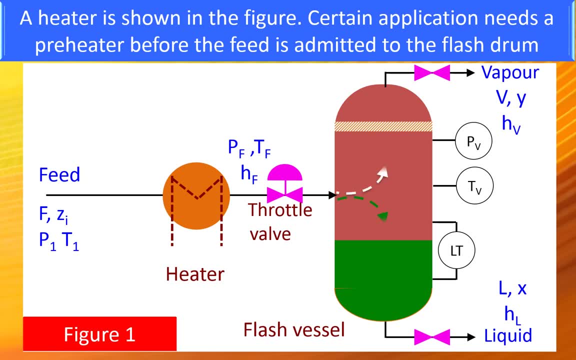 The liquid feed at stated conditions flows through a throttle valve or nozzle to a flash drum. A heater is shown in the figure. Certain applications needs A pre-heater before the feed is admitted to the flash drum. Because of the difference in pressure pot of the liquid vaporizes. 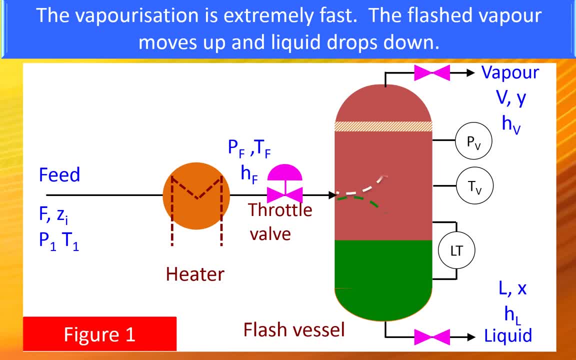 The vaporization is extremely fast. The flash vapor moves up and the liquid drops down. The flash drum provides a sufficient residence time for the flash vapor and liquid to separate. The vapor is removed as overhead, whereas the liquid accumulates at the bottom. 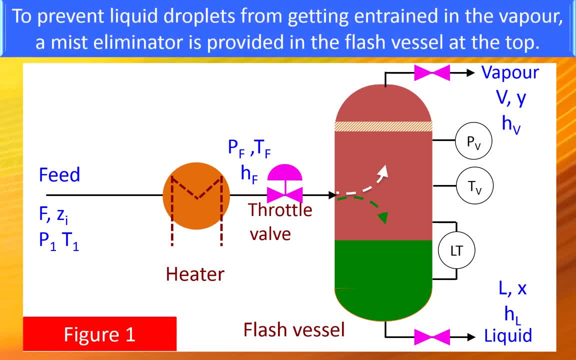 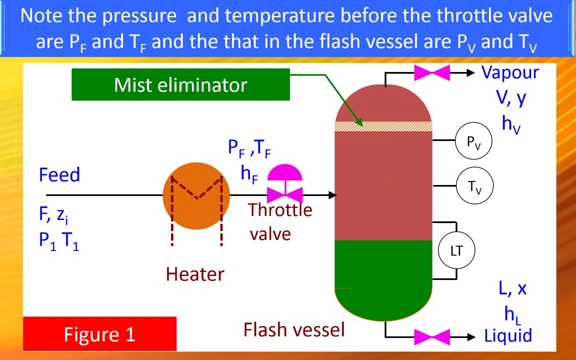 To prevent liquid droplets from getting entrained in the vapor, a mist eliminator is provided in the flash vessel at the top. Note the pressure and temperature before the throttle valve, or PF and TF, and that in the flash vessel, or PV and TV. 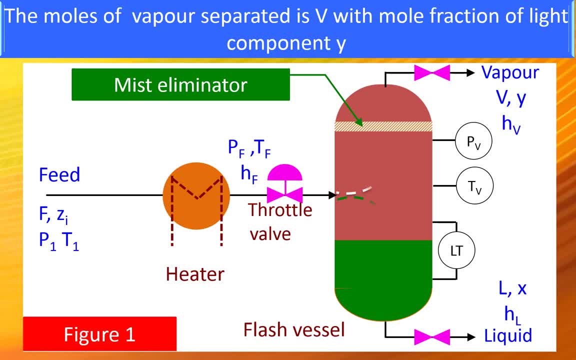 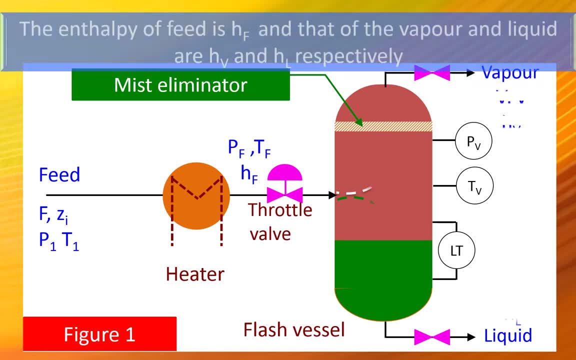 The modes of the vapor separated is V with mole fraction of light component Y, and there are the liquid is L with mole fraction of light component Y. The vapor is separated from the liquid at the top The mole fraction of the light component X. The enthalpy of the feed is HF and there are the vapor and liquid or HV and HL respectively. 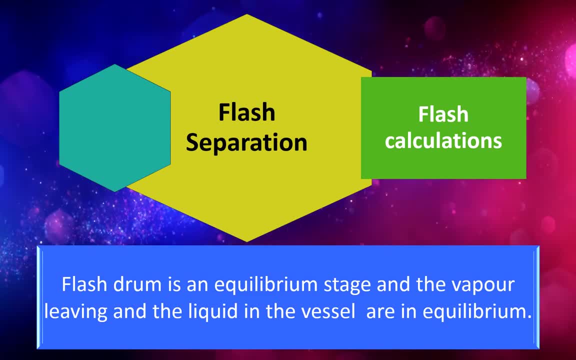 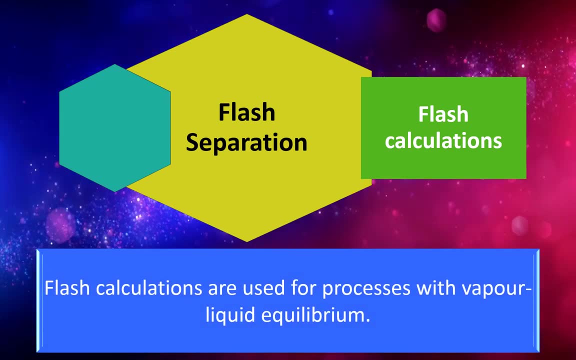 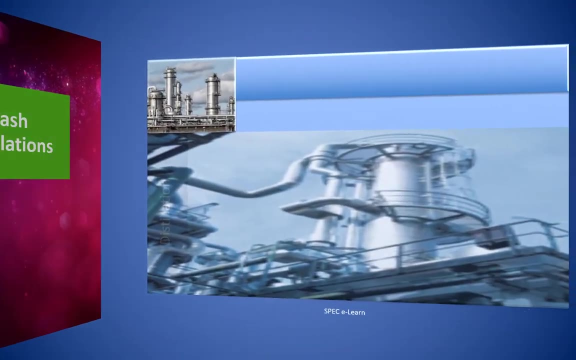 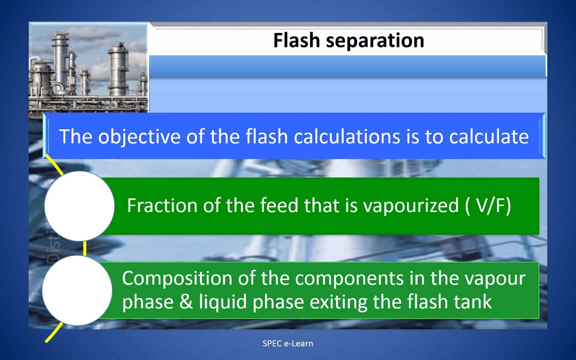 Flash calculations. Flash drum is in equilibrium stage and the vapor and liquid in the vessel are in equilibrium. Flash calculations are used for processes with vapor-liquid equilibrium. The objective of the flash calculation is to calculate the fraction of the fluid that is vaporized, that is, V by F ratio, and the combustion of the components in the vapor. 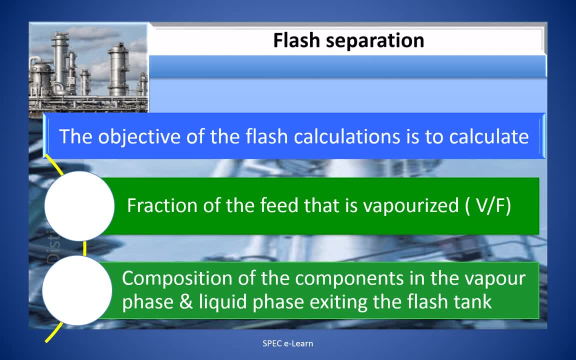 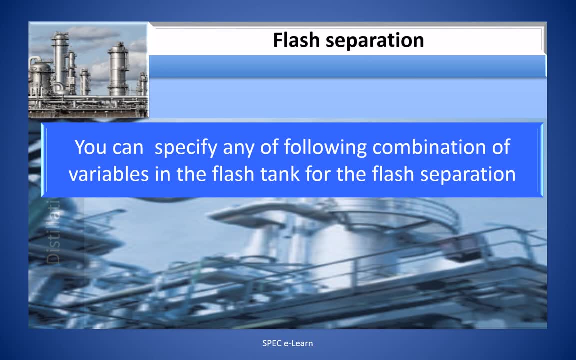 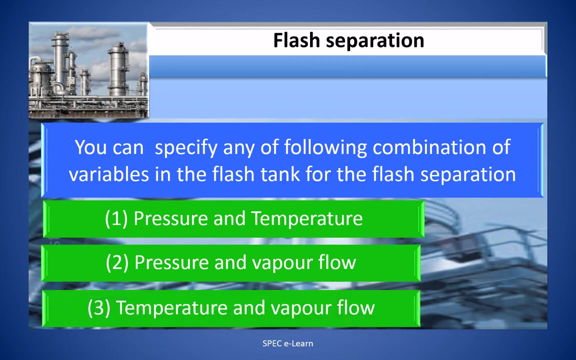 phase and the liquid phase exiting the flash tank thereafter. Next You can specify Subtract. Then R wave against variables in the flash tank for the flash operation: 1. Pressure and temperature. 2. Pressure and vapor flow. 3. Temperature and vapor flow. 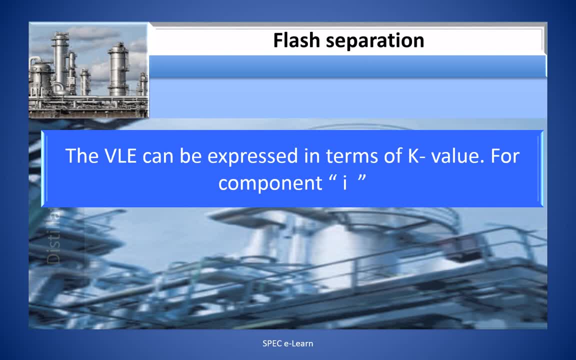 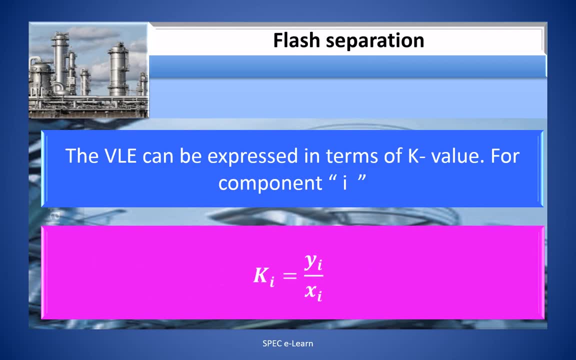 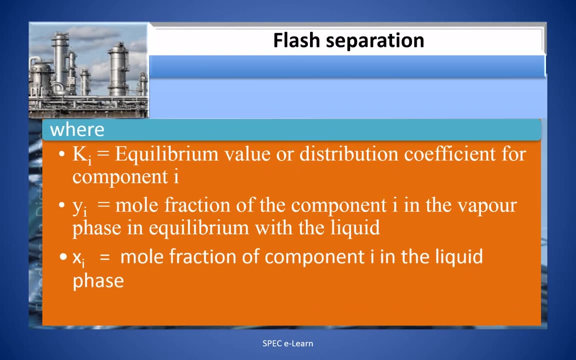 The vapor-liquid equilibrium, VLE, can be expressed in terms of K value For component I: Ki equal to Yi byxi, whereз yi byxi. whereKi is equal to equilibrium value or distribution coefficient. for component II: y is the mole fraction of the component I in the vapor phase. 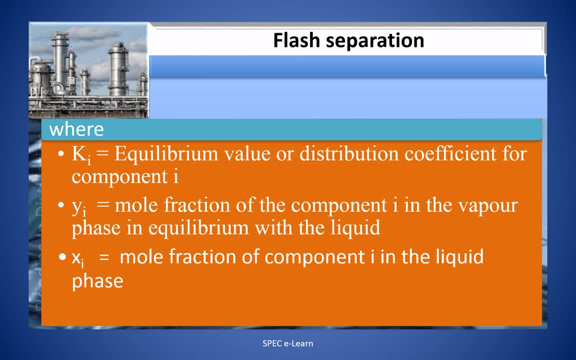 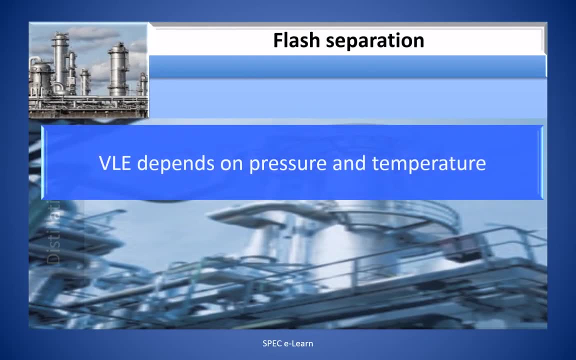 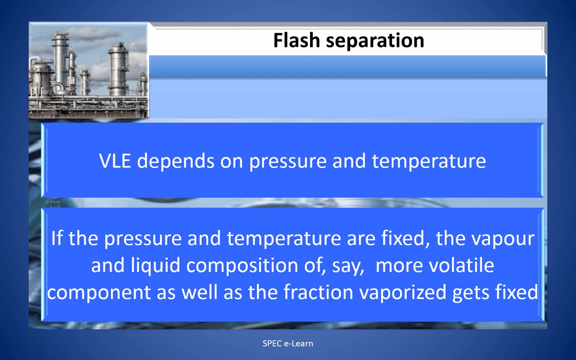 xi is the mole fraction of the component I in the liquid phase. VL depends on the pressure and temperature. If the pressure and temperature are fixed, the vapour and liquid composition of, say, more volatile components, as well as the fraction vaporized, gets fixed. 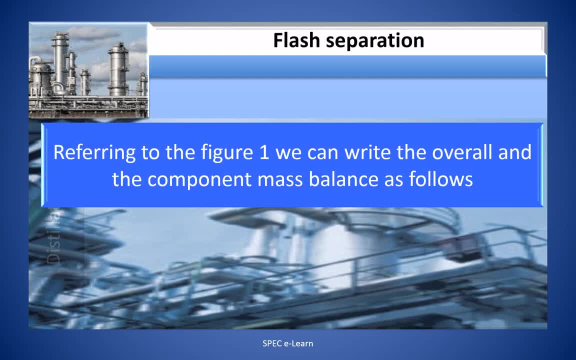 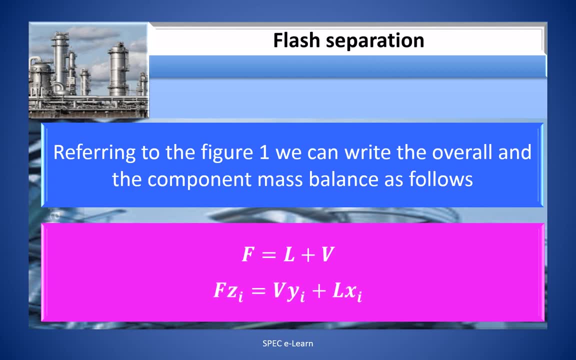 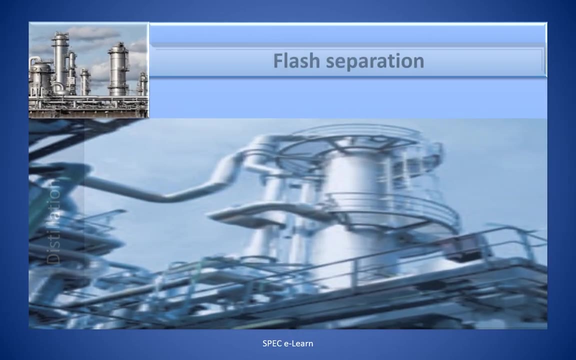 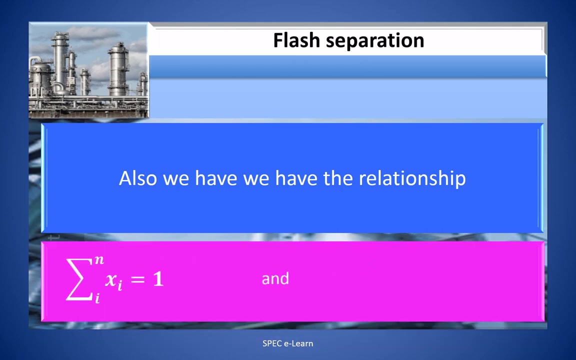 Referring to the figure 1,, we can write the overall and component mass balance as follows: F equal to L plus V and F times Zi equal to V times Yi plus L times Xi. Also, we have the relationship sigma i to n? Xi equal to 1 and sigma i to n? Yi equal to. 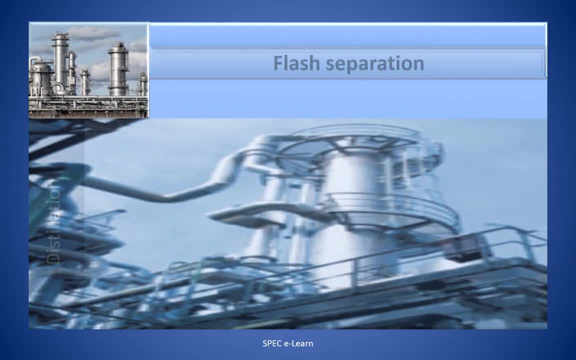 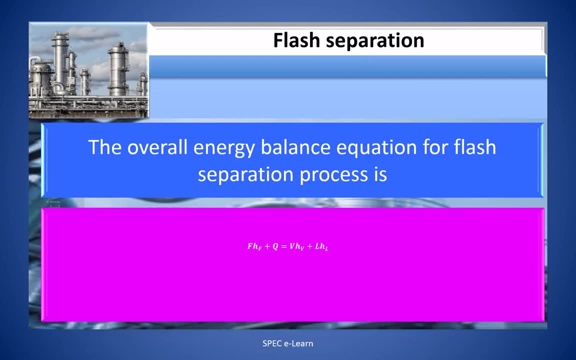 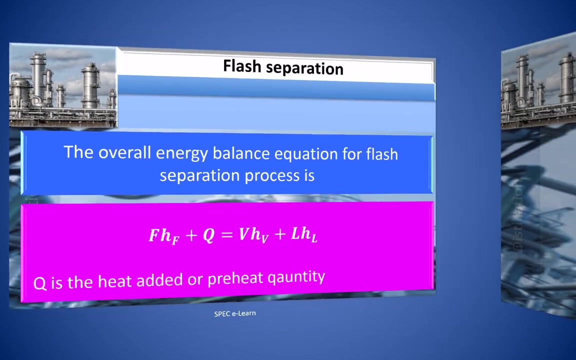 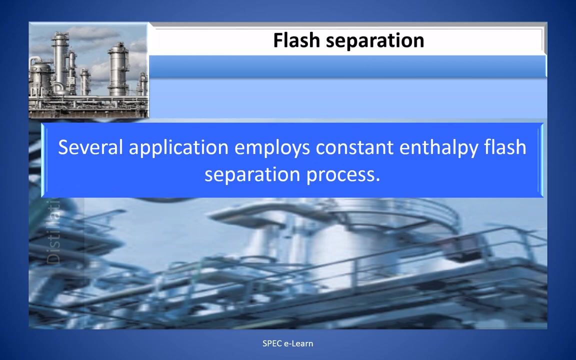 1. The overall energy balance is like this: The energy balance equation for flash separation process is F times HF plus Q, equal to V times HV plus L times HL. Q is a heat added or preheat quantity. Several applications employs constant enthalpy flash separation process. 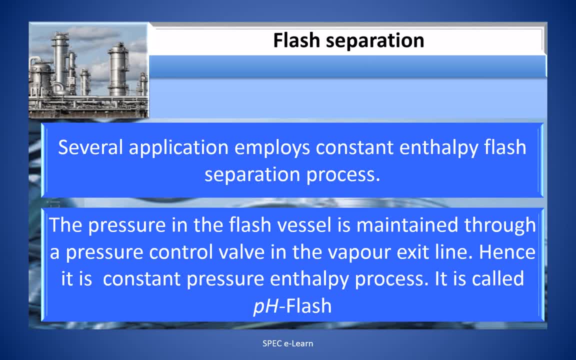 The pressure in the flash vessel is maintained through a pressure control valve. The pressure in the flash vessel is maintained through a pressure control valve. The pressure in the flash vessel is also maintained through a heat control valve. The pressure in the flash vessel is maintained through a heat control valve. 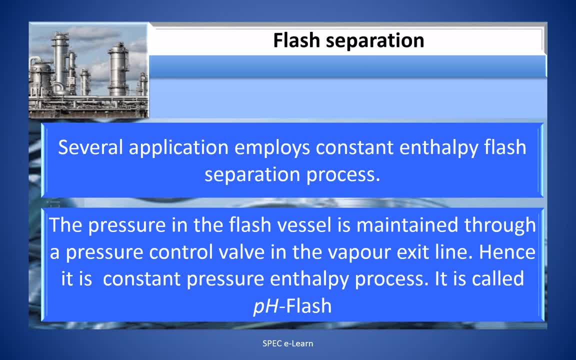 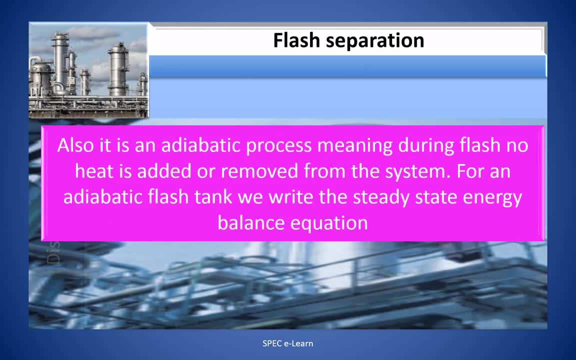 The pressure in the flash vessel is maintained through a heat control valve In the paper exit line, Hence it is constant pressure enthalpy process. It's called PH flash. Also it is an adiabatic process, Meaning during flash no heat is added or removed from the system. 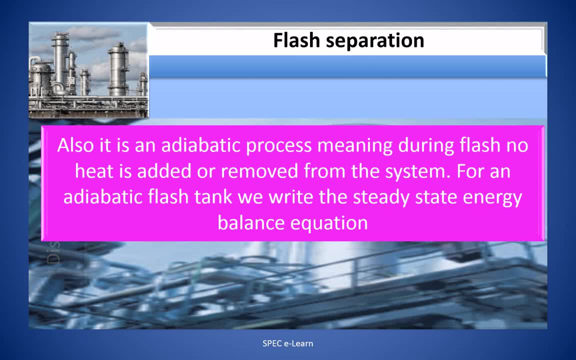 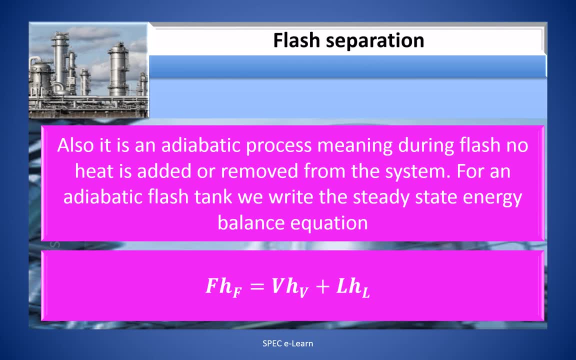 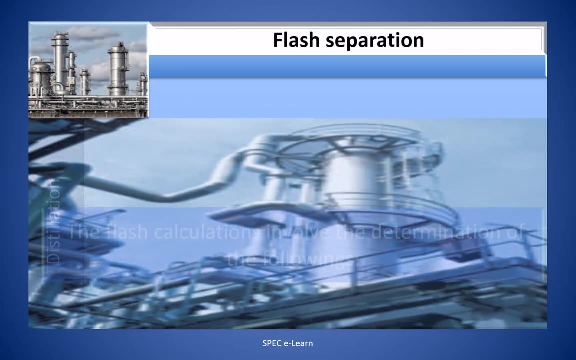 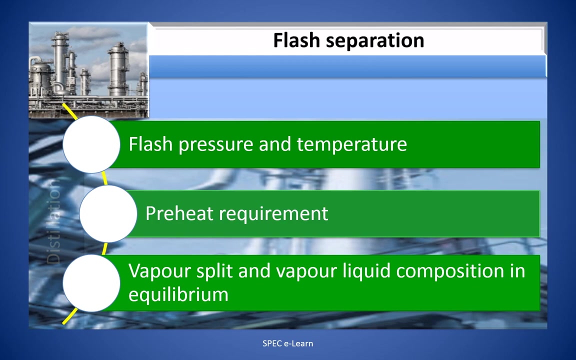 For an adiabatic flash tank, we write the steady state energy balance equation: F times HF equal to V times HV plus L times HL. The flash calculations involve the determination of the following: Flash pressure and temperature, preheat requirement, vapour split and vapour liquid composition. 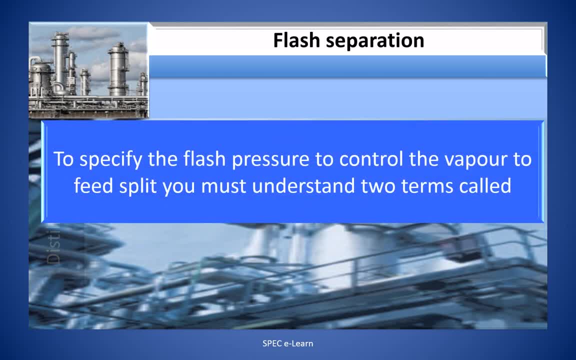 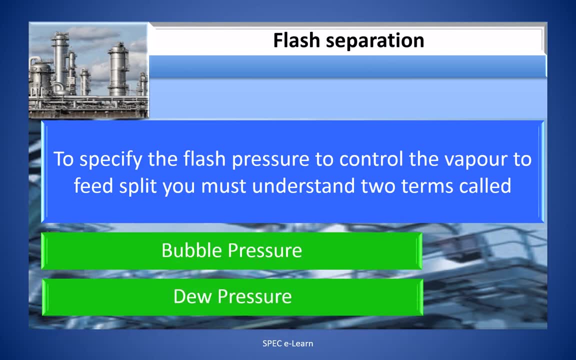 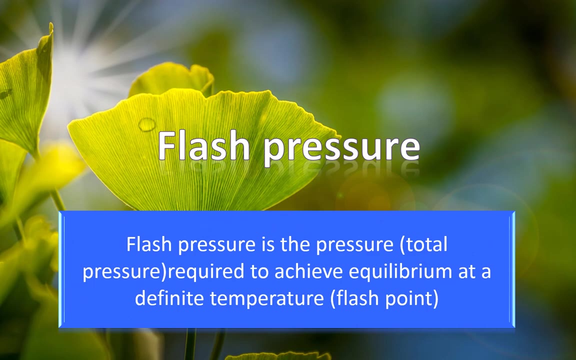 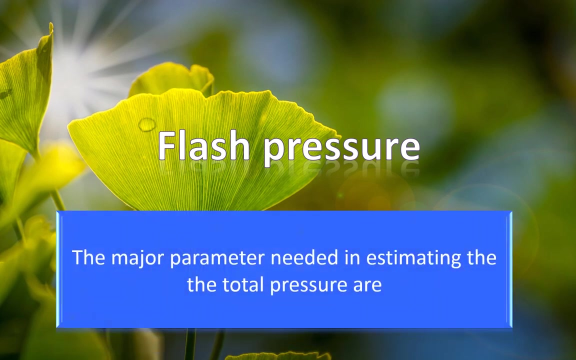 in equilibrium. To specify the flash pressure to control the vapour to feed split, you must understand two terms called bubble pressure and dew pressure. Flash pressure- Flash pressure is the pressure required to achieve equilibrium at a definite temperature. that is flash point. The major parameters needed in estimating the total pressure are: 1- the vapour pressure. 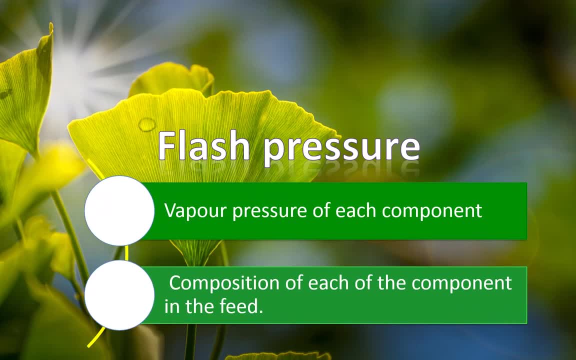 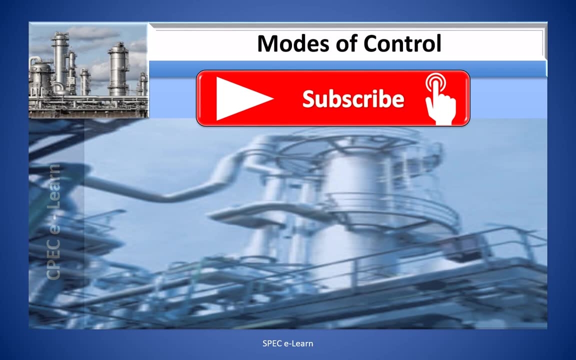 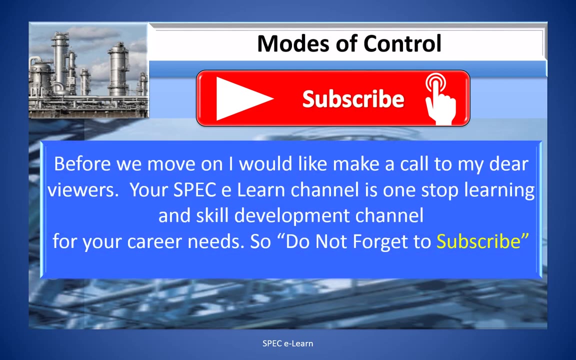 of each component. 2: the composition of each component in the feed. Before we move on, I would like to make a call to my dear viewers. your SPEC Elon channel is a one star channel. Stop learning and skill development channel for your career. 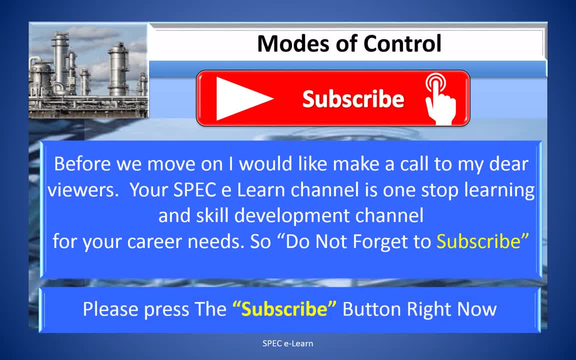 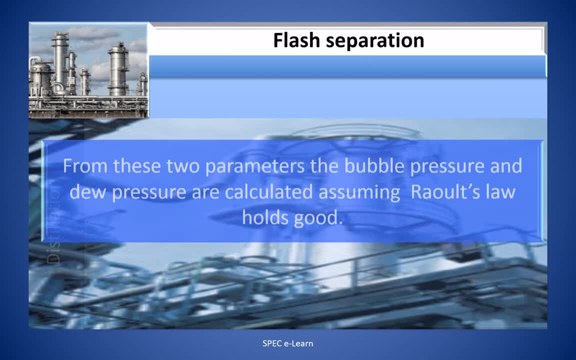 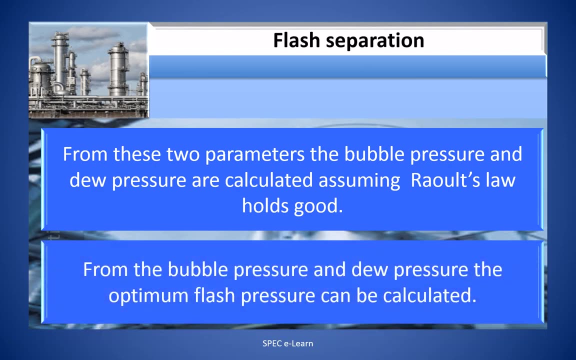 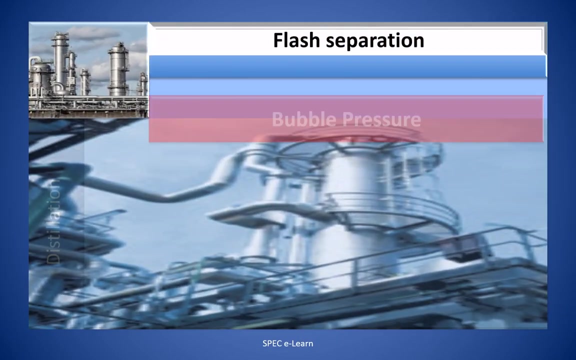 So do not forget to subscribe. Please press the subscribe button right now. From these two parameters, the bubble pressure and dew pressure, are calculated. assuming Routes Law holds good, From the bubble pressure and dew pressure the optimum flash pressure can be calculated. Bubble pressure: 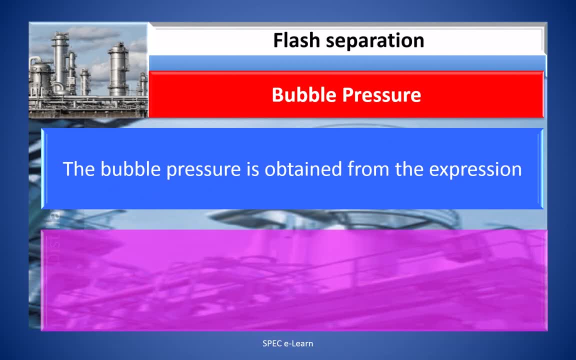 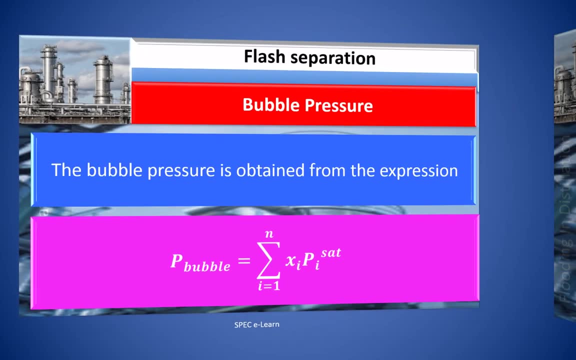 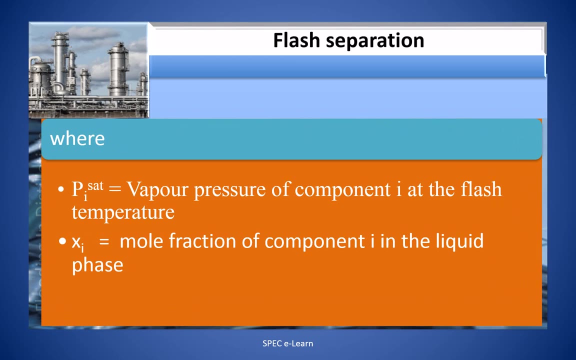 Bubble pressure is calculated from the expression pbubble, equal to sigma i to n, x i times p i sat. where p i sat is the vapour pressure of the component i at the flash temperature x. i is the mole flash that the component in the liquid phase. 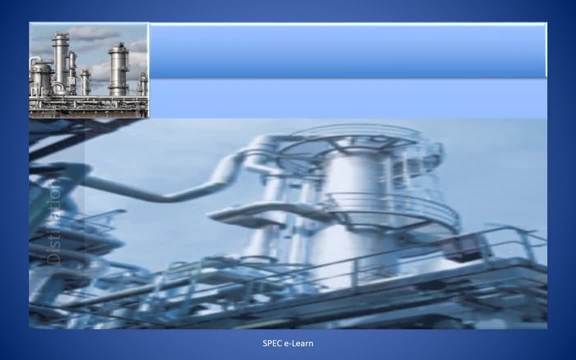 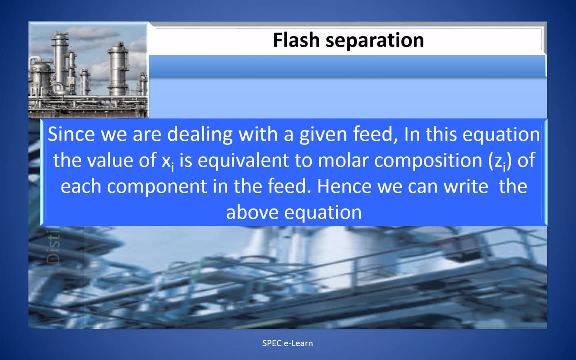 Since the vapor pressure of the component i is the flash temperature. the vapor pressure of the component i is the flash temperature. Since we are dealing with a given feed. in this equation the value of Xi is equivalent to the molar concentration, Zi, of each component in the feed. 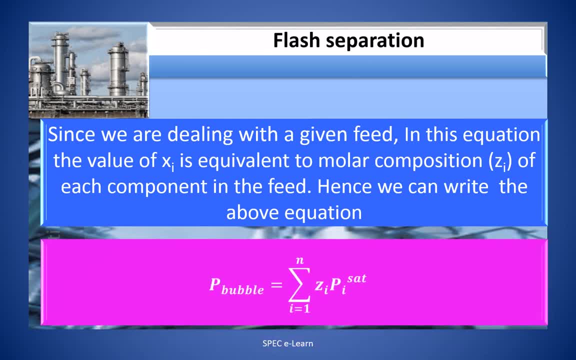 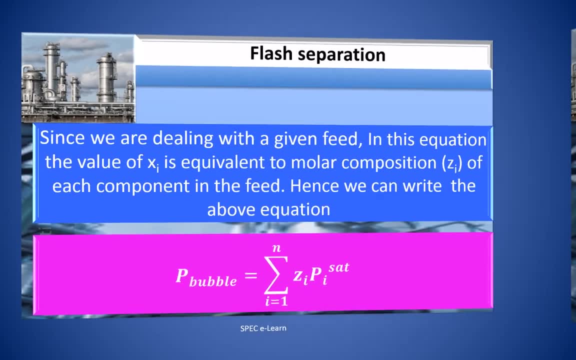 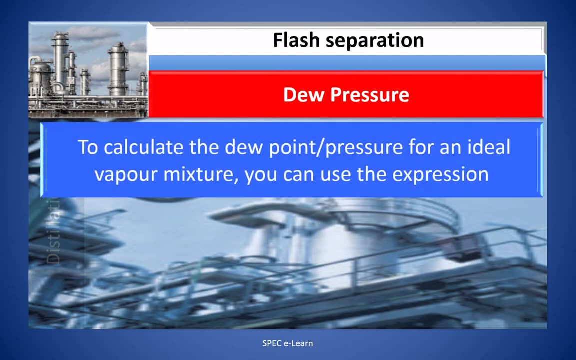 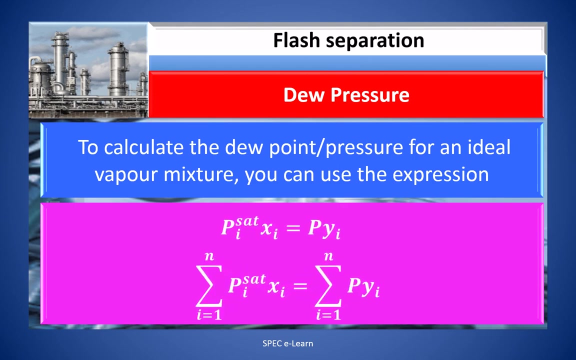 Hence we can write the above equation as: Pbubble equal to Sigma I2n. Zi times PaSat Dew Pressure. To calculate the dew point or pressure for an ideal vapor mixture you can use the expression PaSat times Xi, equal to P times Ya. 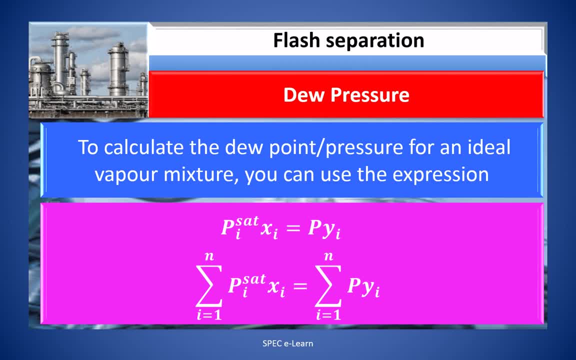 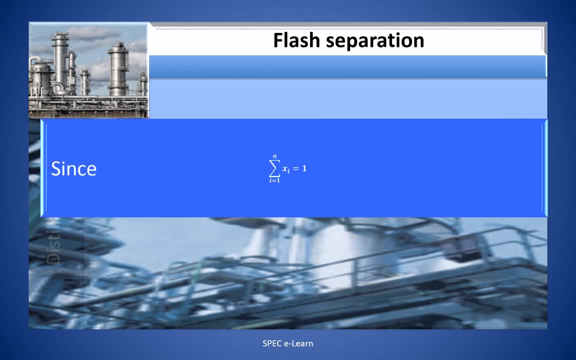 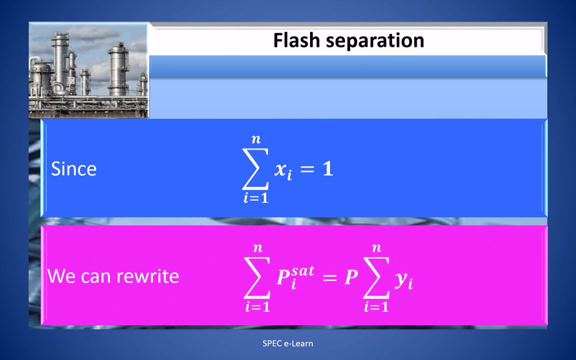 Or Sigma I2n PaSat times Xi equal to Sigma I2n P times Ya. Since Sigm I equal to 1 to n Xi equal to 1.. We can read the following: rewrite: sigma i equal to 1 p i sat equal to p times sigma i to 1 y i. 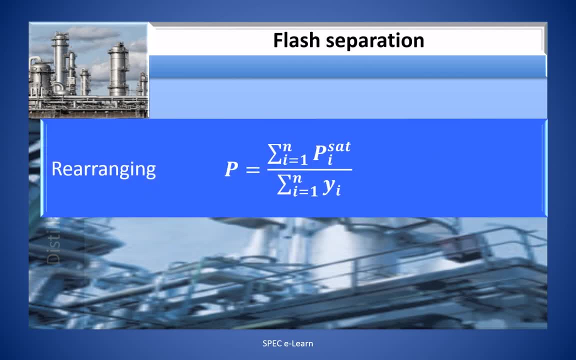 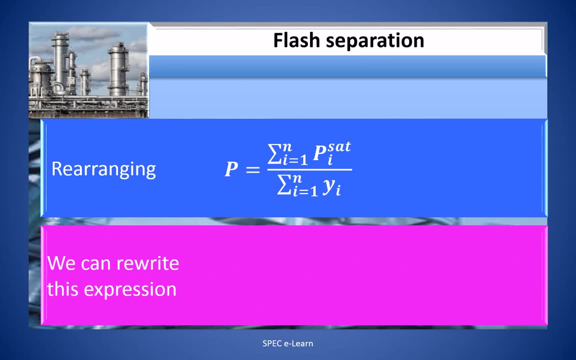 Rearranging we get p equal to sigma i equal to 1 to n p i sat, divided by sigma i. equal to 1 to n y i. We can rearrange this expression as p equal to 1 by sigma i equal to 1 to n y i by p i sat. 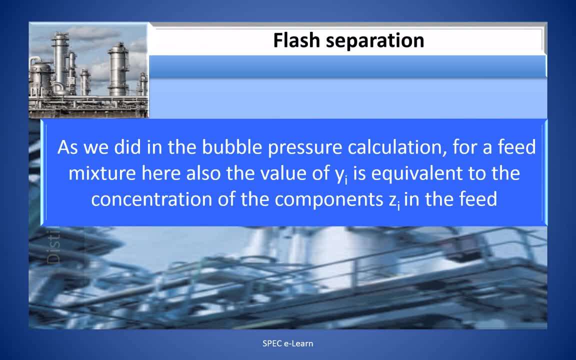 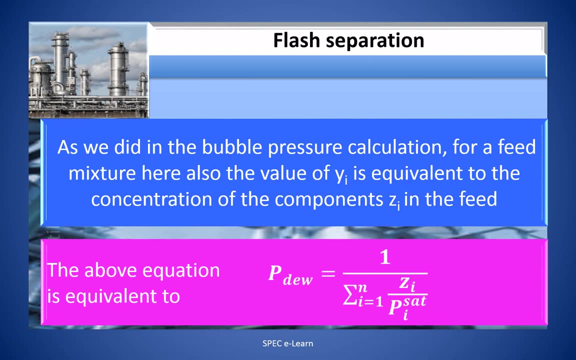 As we did in the bubble pressure calculation for a feed mixer. here also the value of y i is equivalent to the concentration of components z i in the feed. The above equation is equivalent to p div equal to 1 by sigma i equal to 1 to n. z i by p i sat. 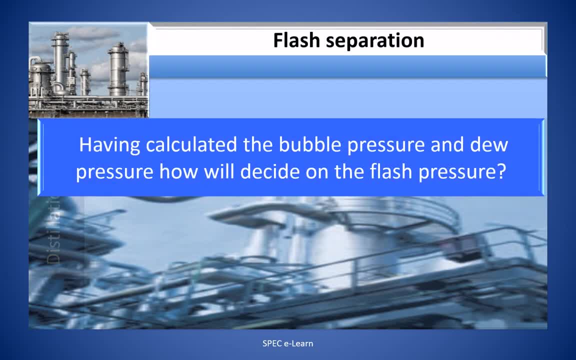 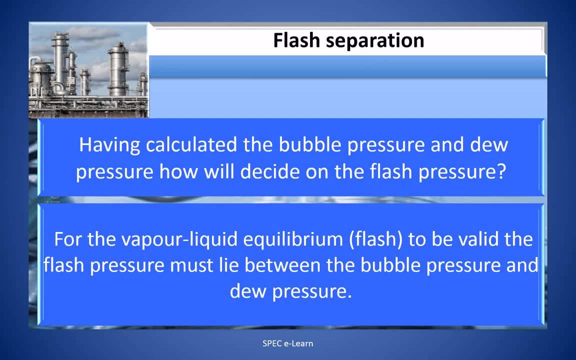 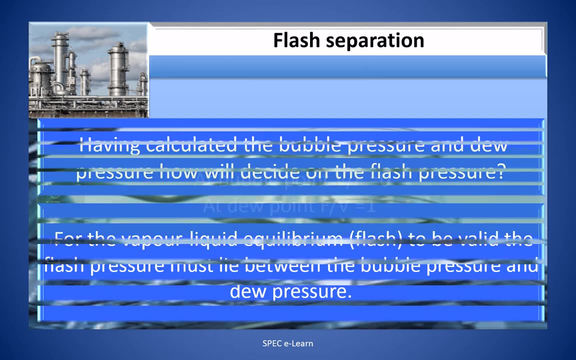 Having calculated the bubble pressure and dew pressure, how will you decide on the flash pressure? For the vapor liquid equilibrium to be valid, the flash pressure must lie between the bubble pressure and dew pressure. At bubble point b by f is equal to 0.. 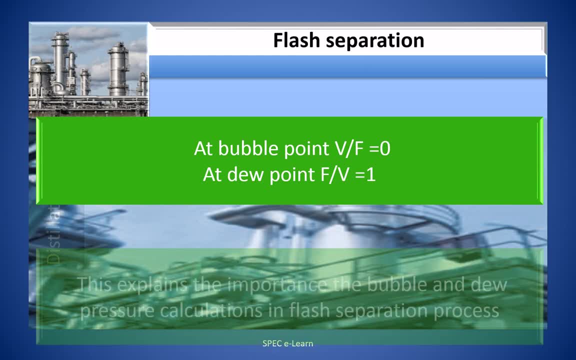 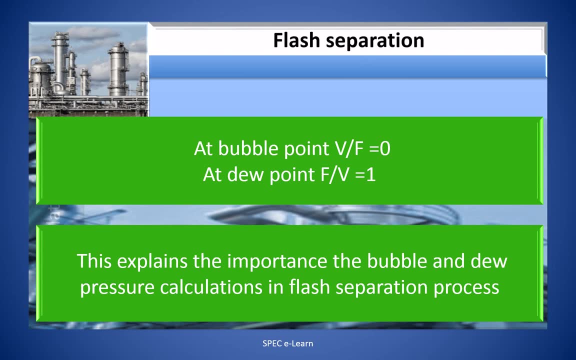 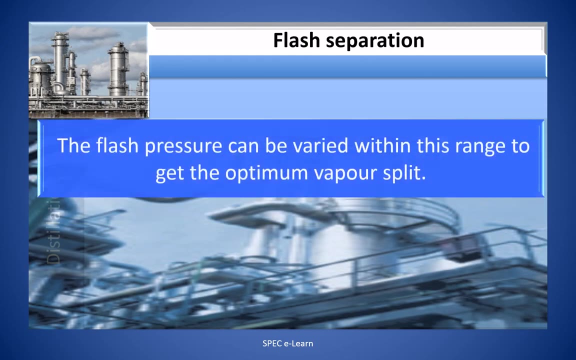 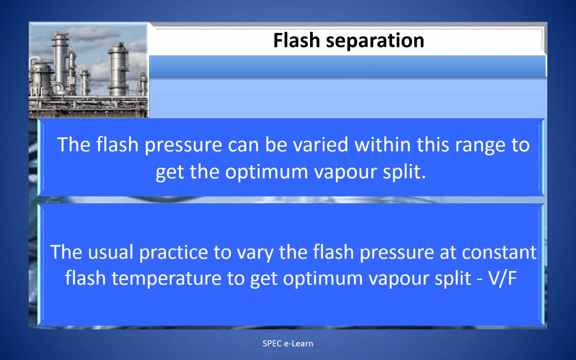 At dew point f by v is equal to 1.. This explains the importance of bubble and dew pressure calculations in the flash separation process. The flash pressure can be varied within this range to get the optimum vapor split. The usual practice is to vary the flash pressure at constant flash temperature to get optimum vapor split. 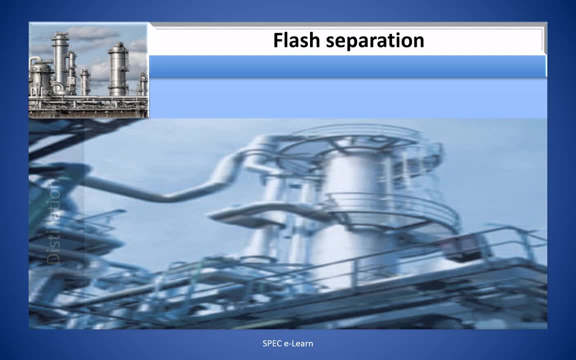 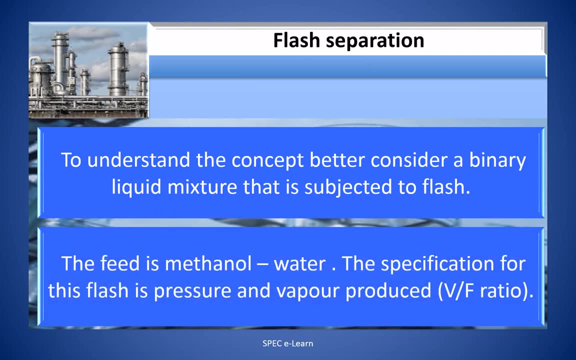 To understand the concept better, consider a binary liquid mixer that is subjected to flash. And now let's look at the droplet at constant velocity, which is at constant Phase. The first is methanol water. The specification for the flash is pressure and vapor produced, ie. 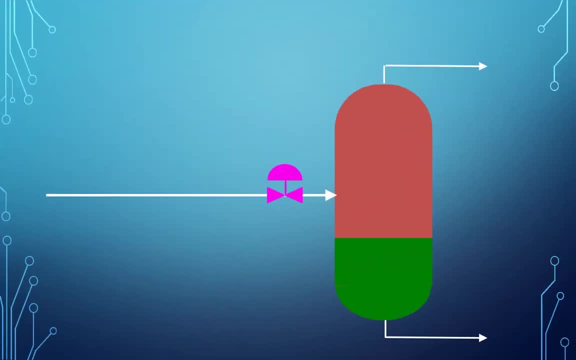 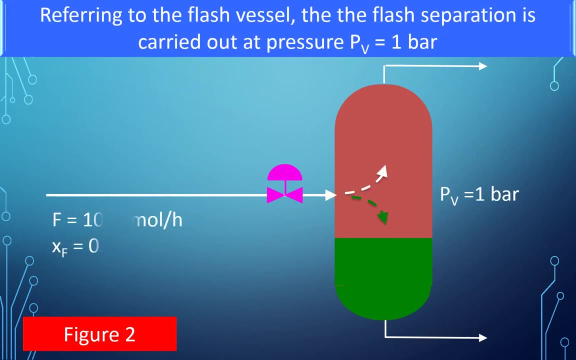 V to f ratio. i Referring to the flash vessel. in this figure, the flash separation is carried out at pressure p v is equal to 1 bar. The feed rate is 100 kmol per hour. The feed concentration of methanol is XF equal to 0.5. 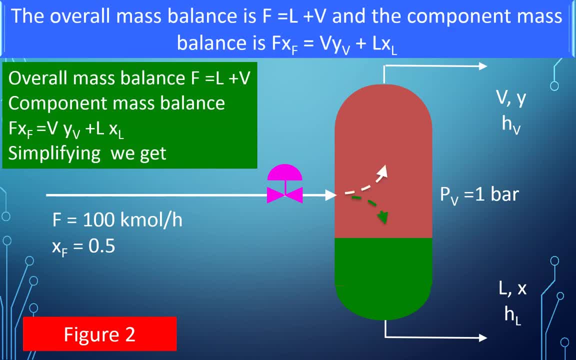 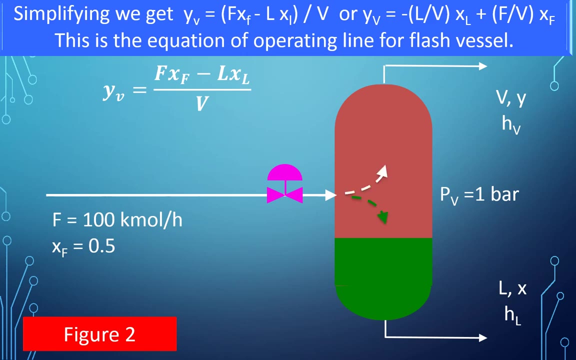 The overall mass balance is Fe濪. The feed rate is 100 kmol per hour, equal to L plus V, and the common mass balance is FxF, equal to VYV plus LXL. Simplifying, we get YV equal to FxF minus LXL divided by V, or YV equal to minus L by V times XL plus F by V times XF. 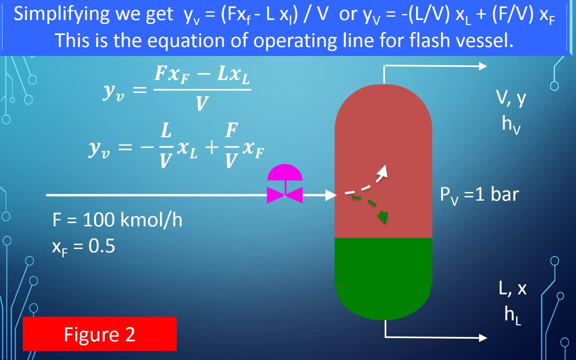 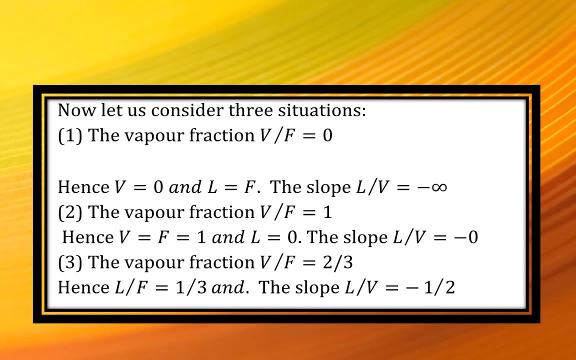 This is equation of operating line for the flash vessel, Minus L by V is the slope of the operating line and F by V times XF is intercept on the McApthelial diagram. Now let us consider three situations. One: the vapor fraction V removed is zero, that is V to F. 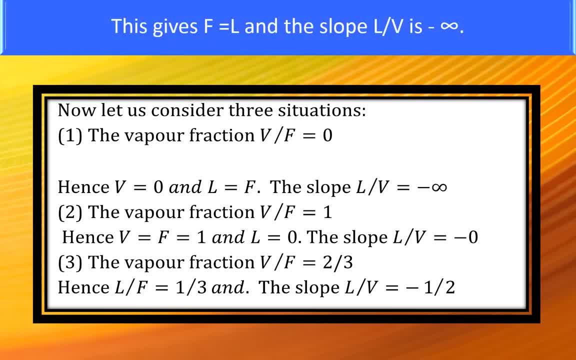 ratio is zero. This gives F is equal to L and the slope L by V is minus infinity. Two vapor fraction V is equal to L and the slope L by V is minus infinity. Two vapor fraction V is equal to L and the slope L by V is minus infinity. 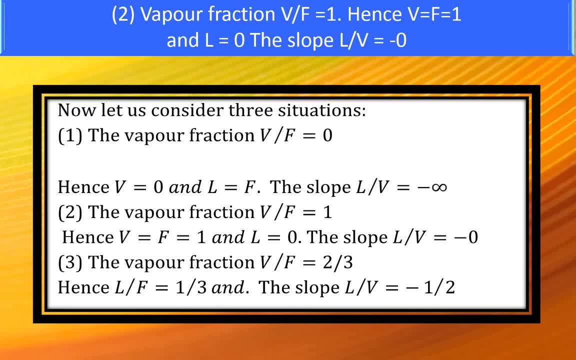 Three: the vapor fraction V to F is 1.. Hence V is equal to F, is equal to 1 and L is equal to 0.. The slope L by V is minus 0.. Three: the vapor fraction V to F is 2 by 3.. Hence L by F is 1 by 3 and the slope of the operating line L by V is minus 1 by 2 or minus 0.5.. 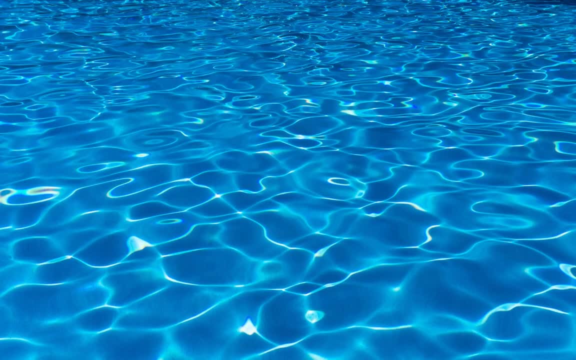 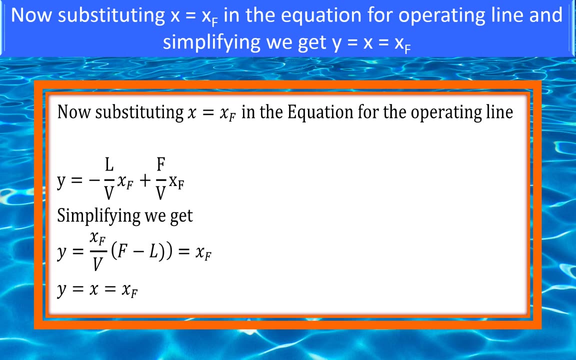 Now substituting X is equal to XF in the equation for the operating line and simplifying, we get: Y is equal to X is equal to XF. That is the feed concentration. XF lies on the diagonal line. In other words, the operating line and the diagonal line intersect at X is equal to XF. 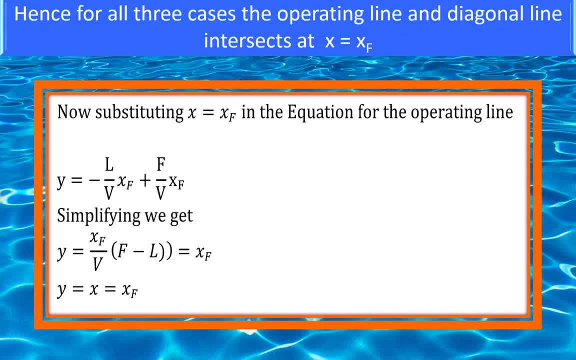 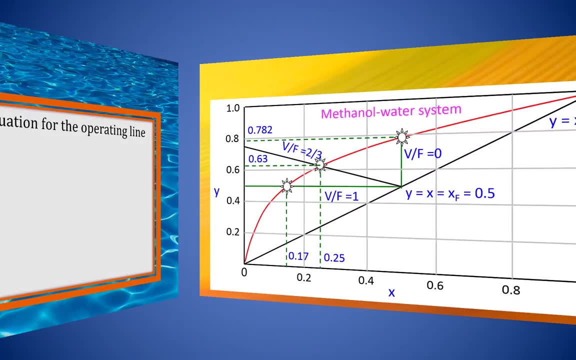 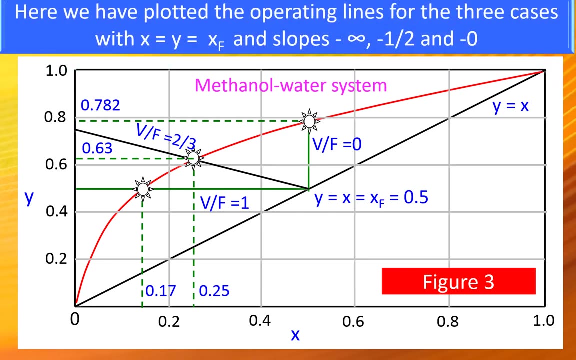 Hence, for all the three cases, the operating line and the diagonal line intersect at X is equal to XF. Shown in this figure is a XY-BLA diagram for the methanol water system. Here we have plotted the operating lines for the three cases, with X is equal to Y is equal to XF and the slopes minus infinity, minus 1 by 2 and minus 0.. 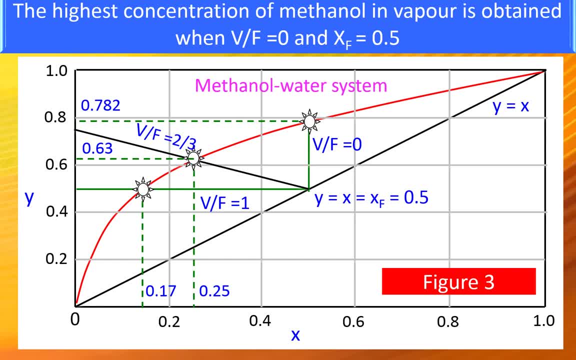 The highest concentration of methanol in the vapor is 0.5.. In the rest it is obtained when V by F is 0 and XF is equal to 0.5.. In this case the operating line cuts equilibrium line at v is equal to 0.782.. 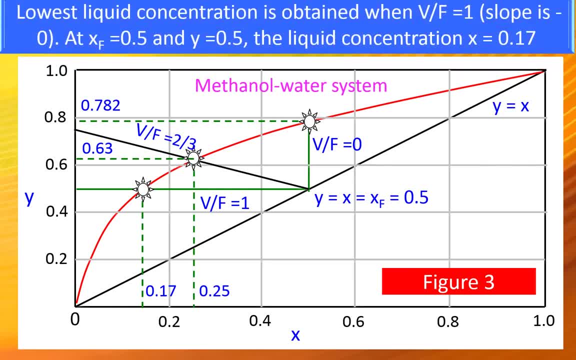 The lowest liquid concentration is obtained when V bygy 0 is 1, that is, slope is minus 0.. At XF equal to 0 point 0 and y is equal to 0.5, the liquids concentration Xu equal to point 1, 7.. 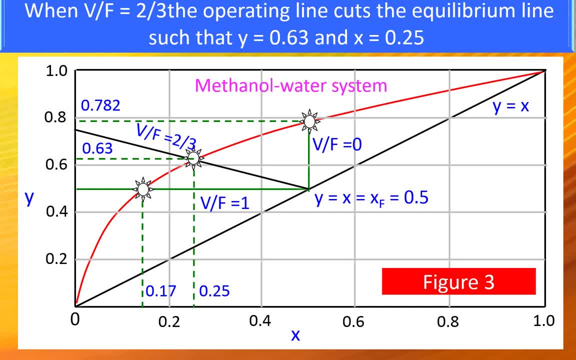 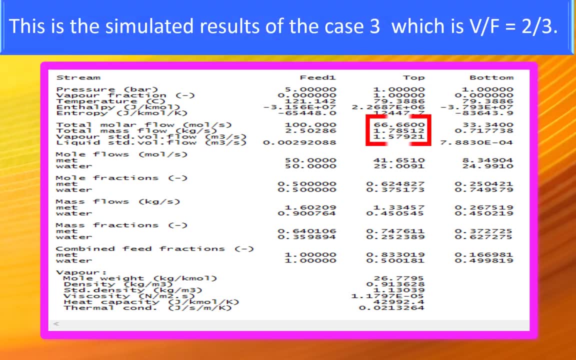 When V by F is 2 by 3, The operating line cuts the equilibrium line such that y is 0.63 and x is 0.25.. This is the simulated results of the case 3, which is B by F is equal to 2 by 3.. 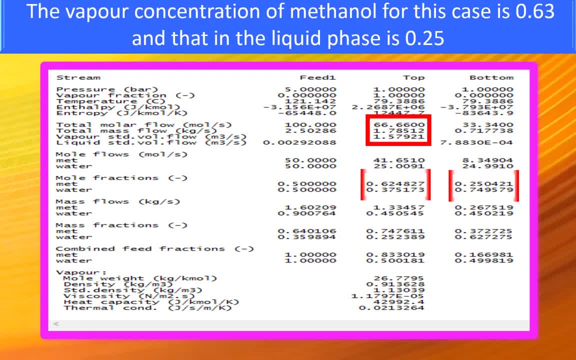 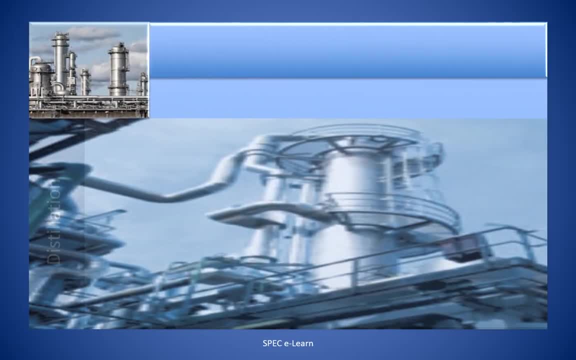 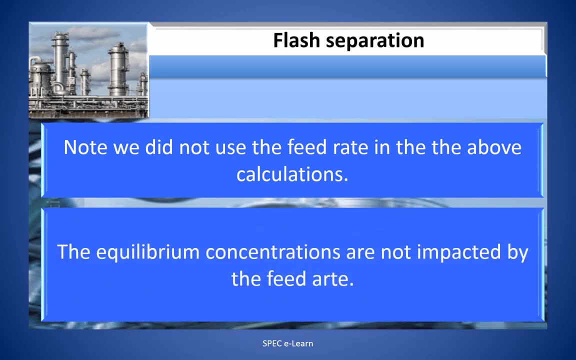 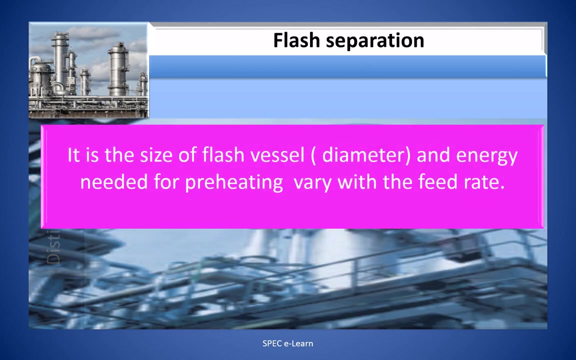 The vapor concentration of methanol for this case is 0.63 and that in the liquid phase is 0.25.. Note: we did not use the feed rate in the above calculations. The equilibrium concentrations are not impacted by the feed rate. It is the size of the flash vessel. diameter and energy needed for preheating vary with. 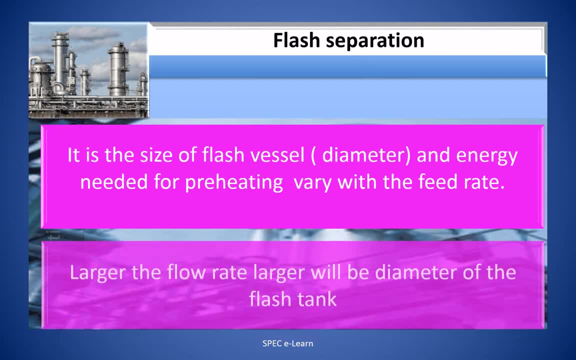 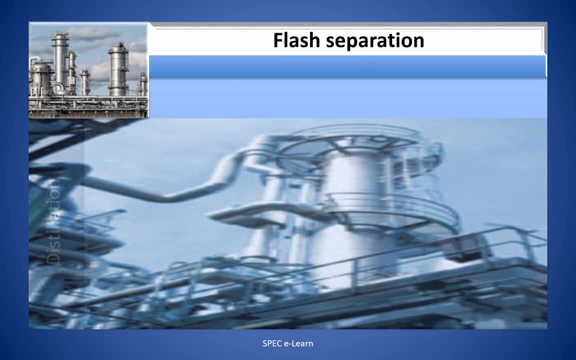 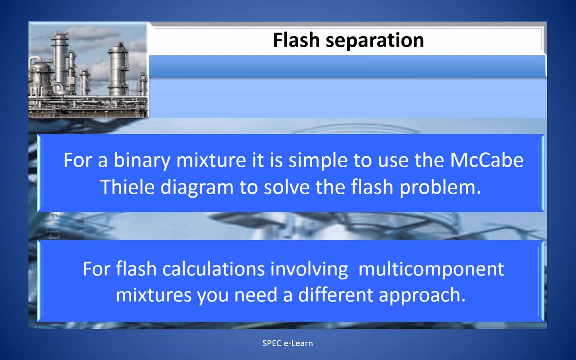 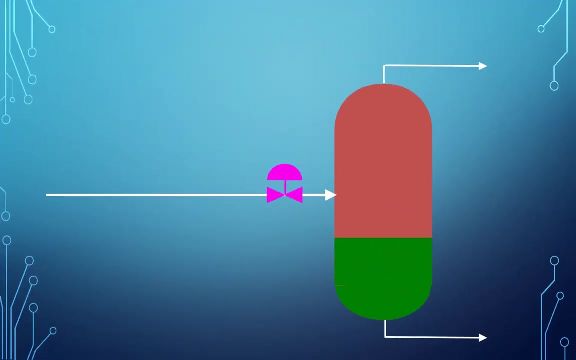 the feed rate. Larger the flow rate, larger the diameter of the flash tank. For a binary mixer it is simple to use a makepthelia diagram to solve the flash problem. For flash calculations involving multi-component mixes you need a different approach. 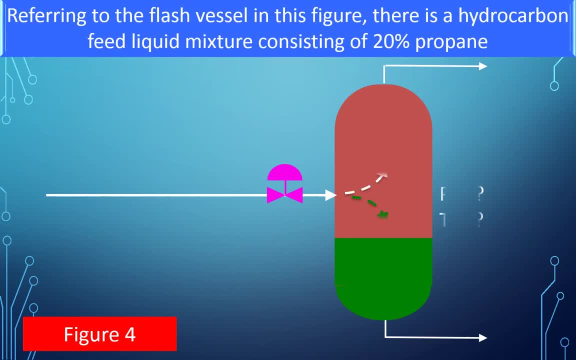 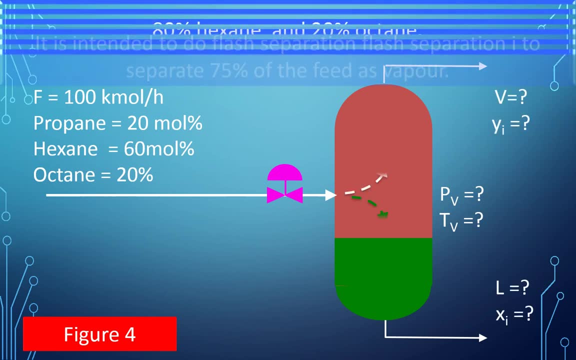 Referring to the flash vessel in this figure. there is a hydrocarbon feed liquid mixer consisting of 20% propane, 80% hexane and 20% octane. It is intended to do flash separation. It is intended to do flash separation. 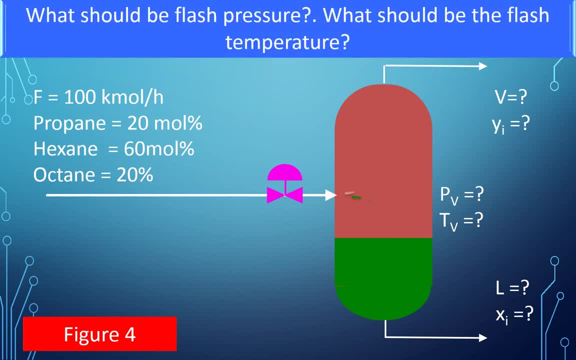 To separate 75% of the feed as vapor. What should be the flash pressure? What should be the flash temperature? What be the composition of the vapor stream and liquid stream exiting the tank? These are the interesting calculations you are requested to do in multi-component flash. 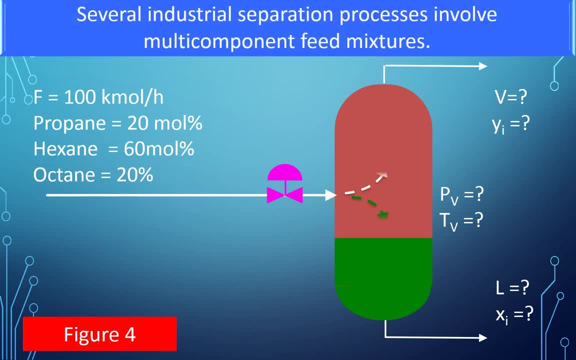 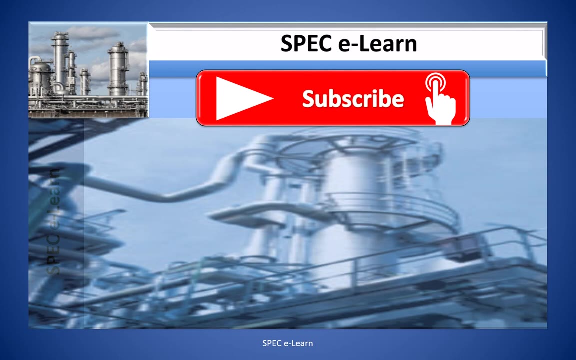 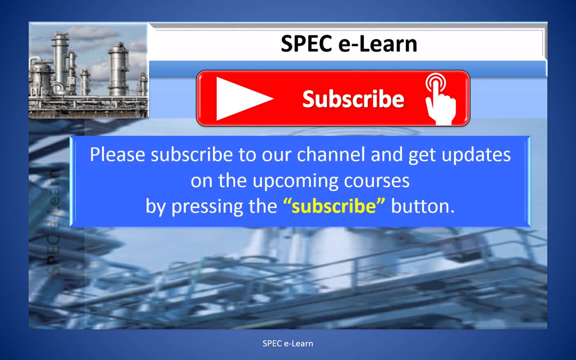 separation: Several industrial separation processes involve multi-component feed mixes. We will cover it in the next video, So do not miss the part 2 of this video. Please subscribe to our channel and get updates on the upcoming courses by pressing the subscribe button. 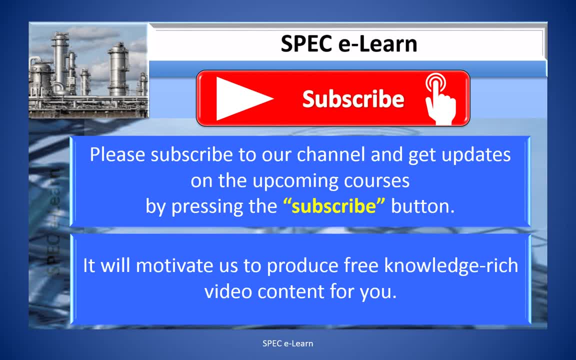 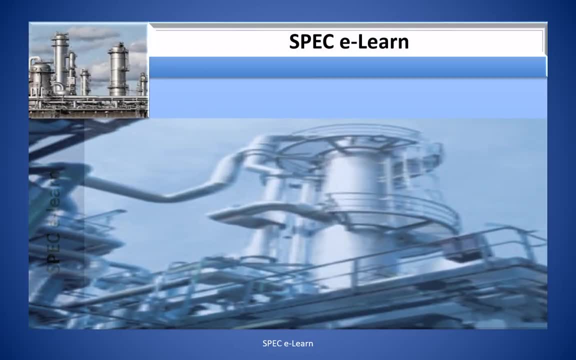 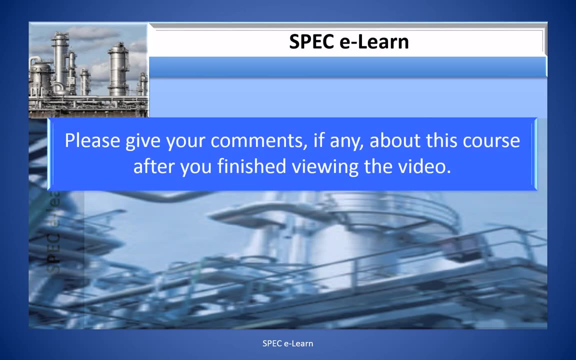 It will motivate us to produce free knowledge, rich video content for you. With this, we have come to the end of the presentation. Please give a comment if you have any questions. Thank you, Thank you, Thank you, Your comments, if you have comments, if any, about this course after you have finished.